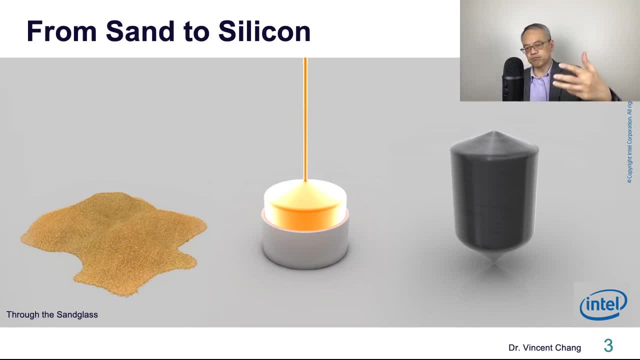 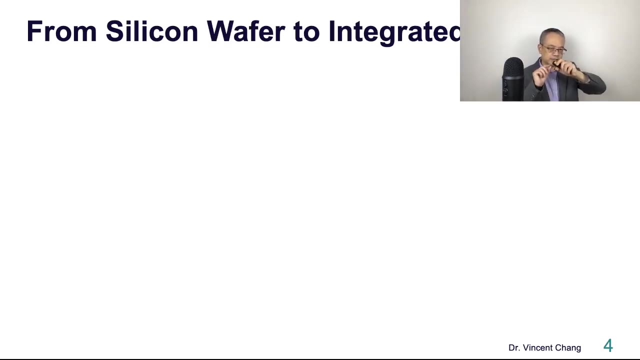 In the middle is the semiconductor fabrication process. On the right is the silicon ingot, Silicon ingot, The pure silicon ingot, And then from silicon wafer. if you cut the ingot then it's a wafer, Then it becomes the wafer. 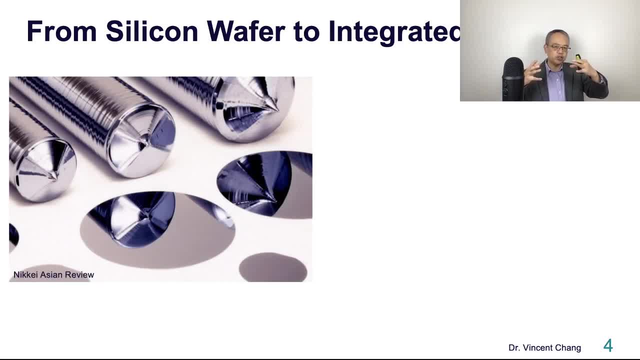 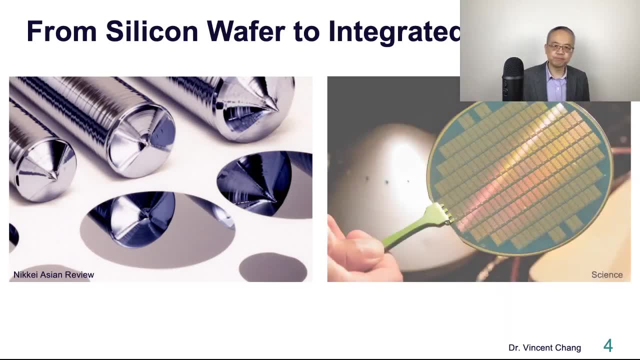 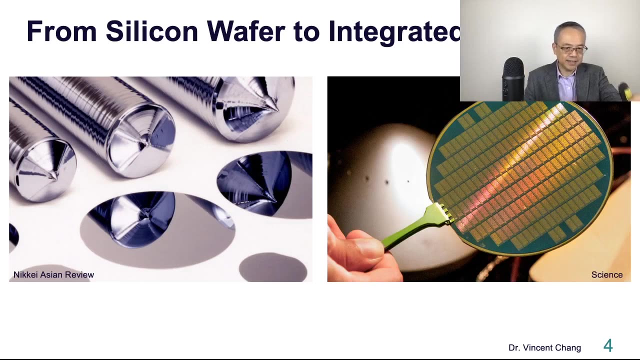 The wafer could be a 6 inch, 8 inch wafer or 12 inch wafer, 300 millimeter wafer diameter, And then it becomes the front silicon wafer on the left to. it's called IC, An integrated circuit. 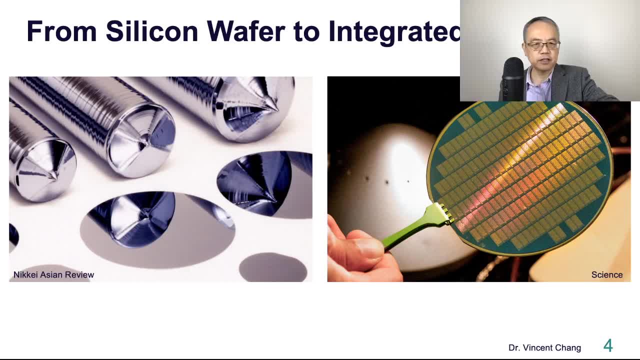 An integrated circuit The different types of electronic component, let's say the resistor, capacitor, inductor, bipolar junction transistor, dial or metal oxide, semiconductor, field effect transistor, all integrated in a small chip, So it's called integrated circuit. And then from IC chip, the integrated circuit chip, to a circuit board. 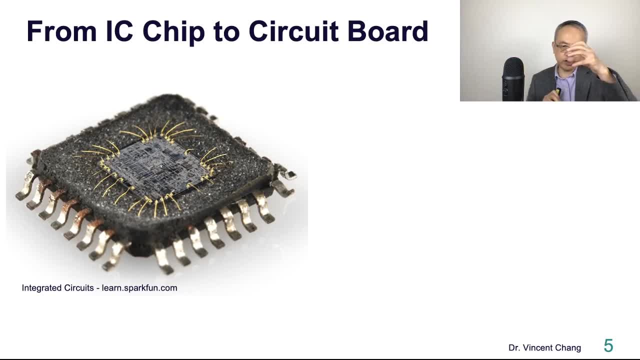 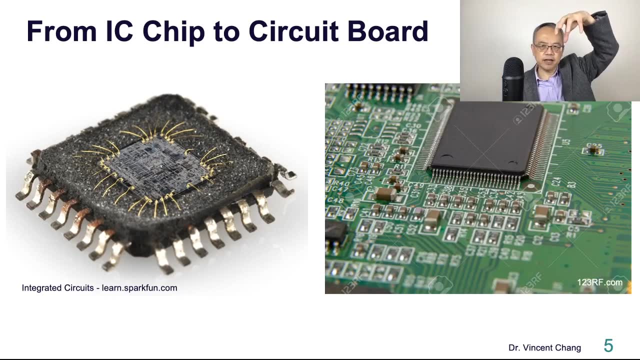 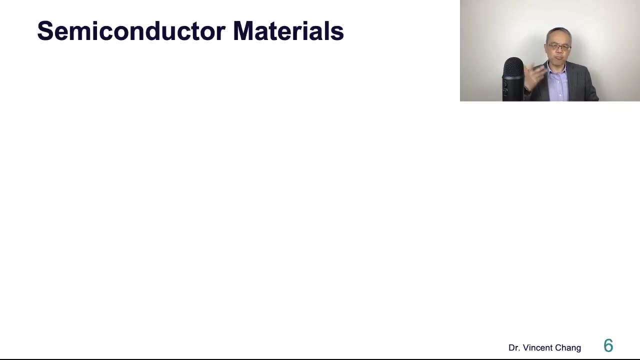 On the left hand side is a chip. You see, the chip is mounted, connected to the pin of a chip. On the right hand side is the chip on a circuit board. So for the semiconductor material, the point I want to make is the several slides from the sand. 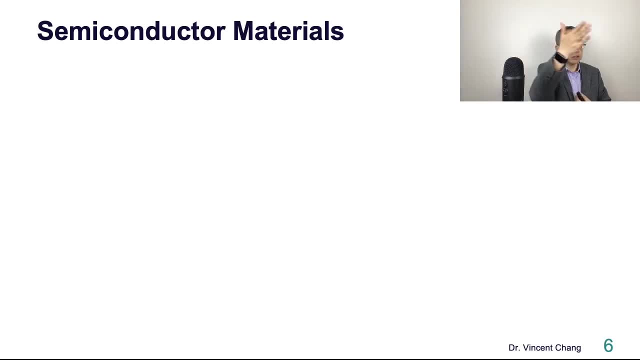 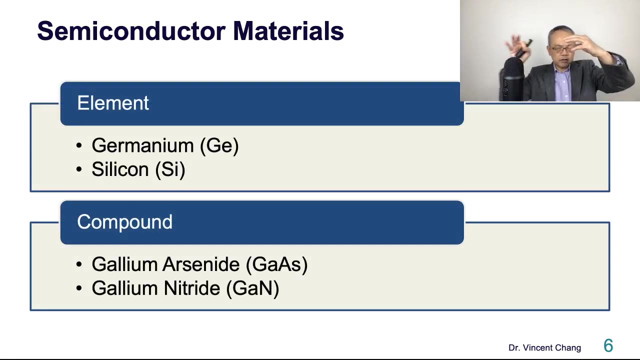 to silicon And from silicon to integrated circuit And from an IC chip to a circuit board. So the underlying material behind this technology is silicon. But if you look at the big picture of about the semiconductor material, you can classify it into two big categories. 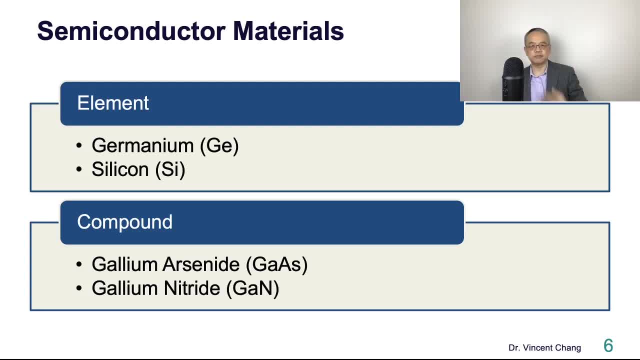 The first is the element semiconductor. The second category is the compound semiconductor. So remember this: The semiconductor material can be grouped into two big categories: Element semiconductor and compound semiconductor, The two most famous element semiconductor materials. the first one is germanium. 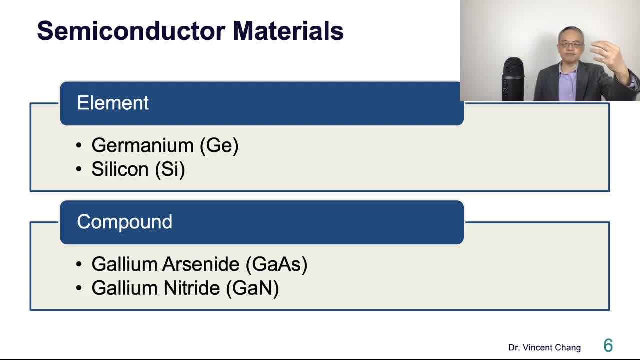 And then the next one is silicon. It's all in the element semiconductor material category, But in the compound category let's say the gallium and arsenate. So it's called gallium arsenide, And then gallium and the nitrogen can form a compound called gallium nitride. 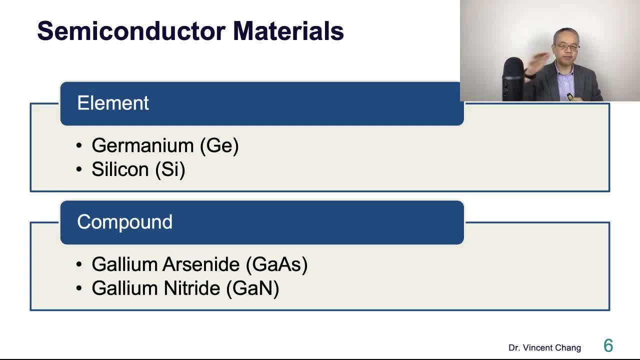 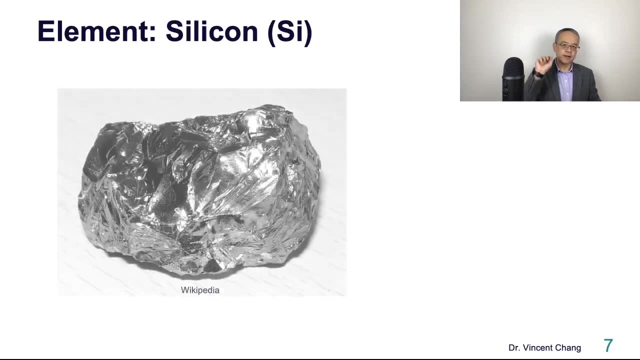 So gallium arsenide. So gallium arsenide and gallium nitride also belongs to the category of the compound semiconductor Element and the compound. Let's start with the element semiconductor, silicon. So silicon valence electron is four. On the left-hand side is the native silicon material. 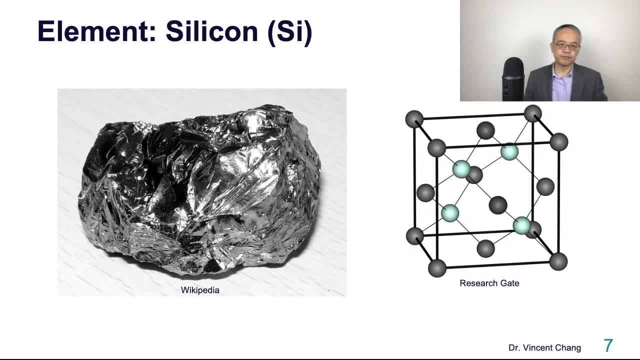 The crystal structure, Crystal structure If you take out the four, the four green ball right, Green atom. So it's called phase phase. There's a center right. It's called phase center qubit And the number of this phase center qubit within a qubit is four. 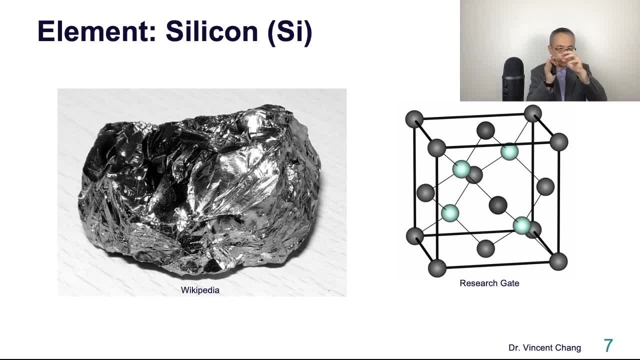 The number of atoms located within, because you can count the six phases and the eight corners right. Eight is one. eighth times eight is one And six phases is half. So half times six is three. One plus three is four If you add another group of four and intersect with each other. 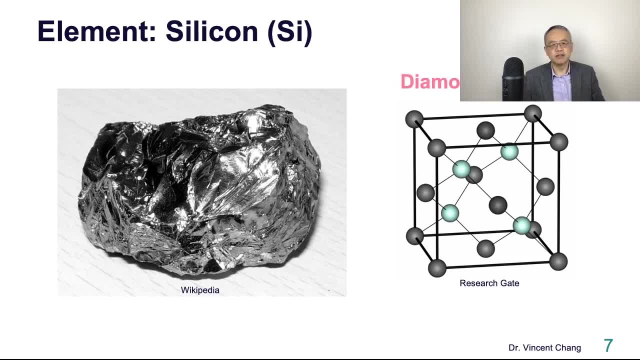 another phase, center qubit. it becomes the crystal structure of the silicon We call the diamond, it's called diamond structure, The crystal crystal structure of the silicon, as diamond is called diamond structure, which is which consists of the two phase center qubit structure. 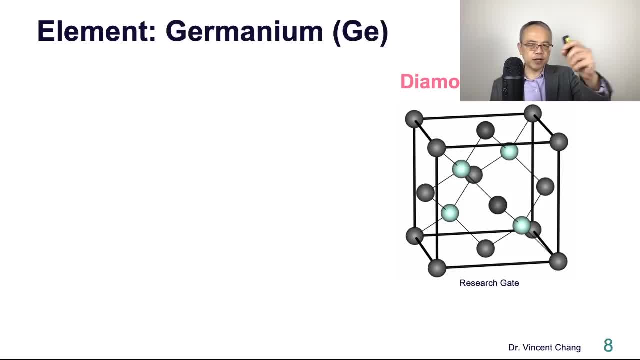 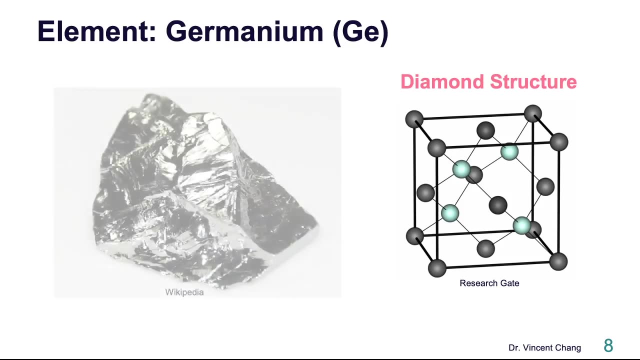 Crystal structure of silicon, But same thing with germanium. It's the same structure for the germanium. Germanium also they are. germanium also belongs to this category. the diamond structure On the left hand side is the native germanium material. 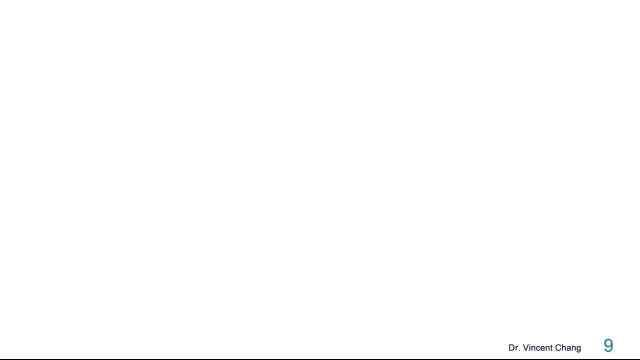 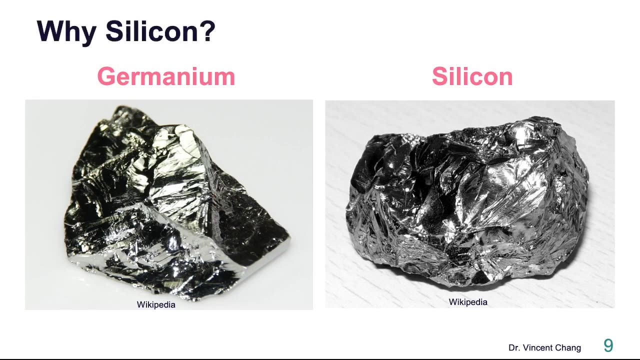 but it's quite expensive. It's quite expensive. So on the left hand side is germanium, on the right hand side is silicon. So why silicon? Why not germanium valley? Why it's called silicon valley? Several reasons. Well, number one: 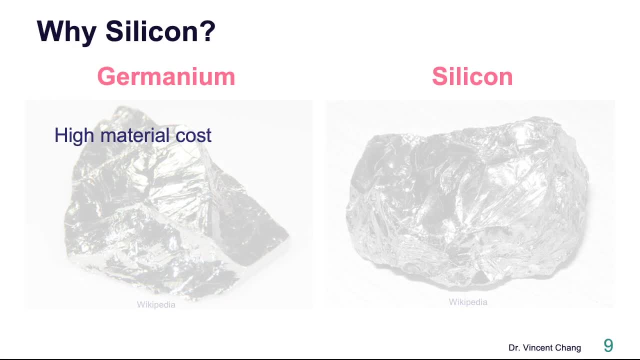 as I just mentioned, germanium is very. the cost is very high, Very expensive. If you want to get pure germanium, it's very expensive, High material cost. Number two: it's a low band gap. I will teach you this in the upcoming lecture video. 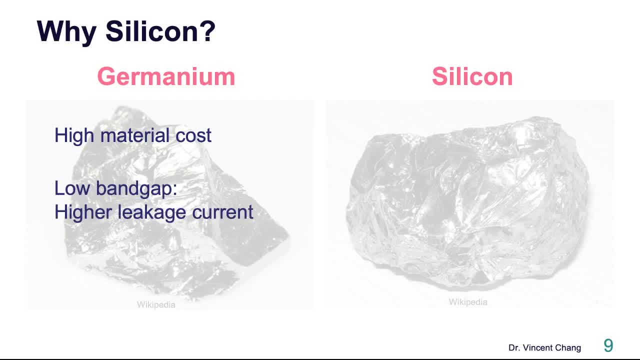 What's the band gap? What's the definition of band gap? But it's the low band gap. But if the material has the low band gap when it comes to leakage current, the leakage current will be high. So low band gap and higher leakage current for device is no good. 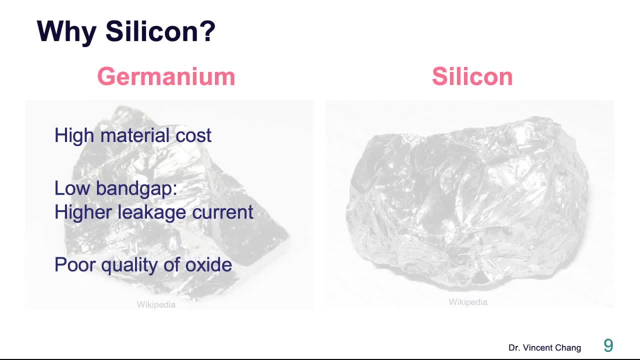 And germanium. if you, germanium, want to want the oxide to be grown out of the germanium material, the quality from the germanium, the germanium oxide, no good quality, No good quality. But on the right hand side is the silicon. 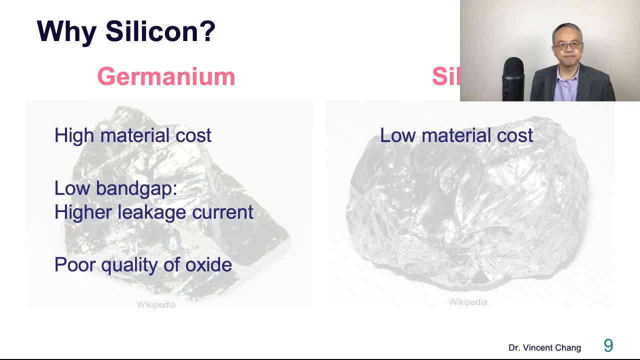 For the silicon low material cost. Low material cost, It's cheap. Okay, The earth is full of silicon, From sand right From sand to silicon. Say it's cheap. And then it's the higher band gap compared to the germanium. 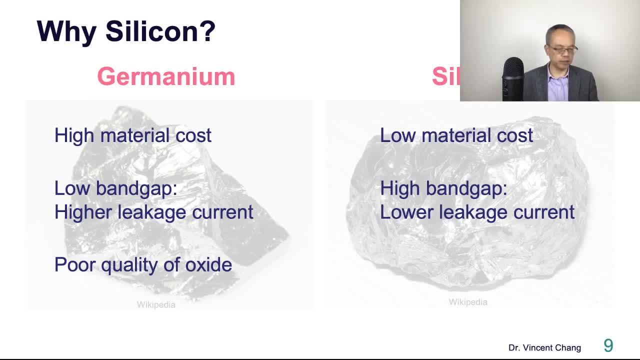 So higher band gap, lower leakage current. The leakage current is much lower compared to the germanium device. And then the last one is very expensive. It's superior quality of silicon dioxide. So one silicon atom and if you come with the two oxygen atoms, 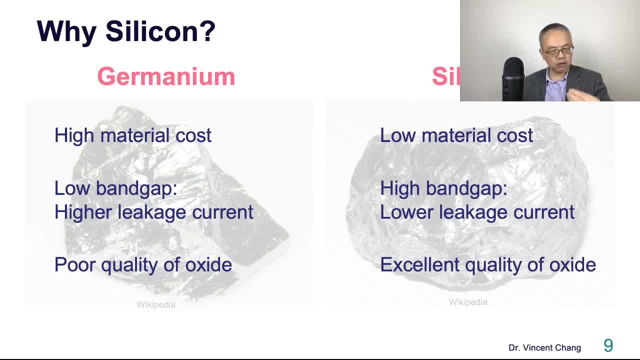 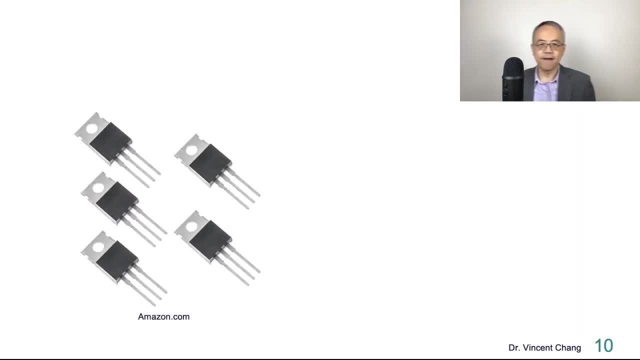 it will form the glass. It's the silicon dioxide, Superior quality of silicon dioxide. And for this, why does this matter? Why oxide matters? For this device it's called. it's a very important electronic device called MOSFET. 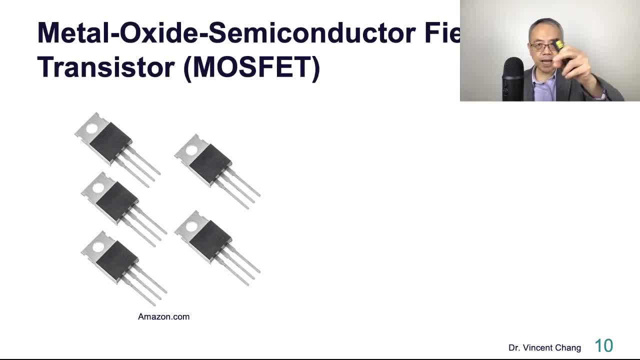 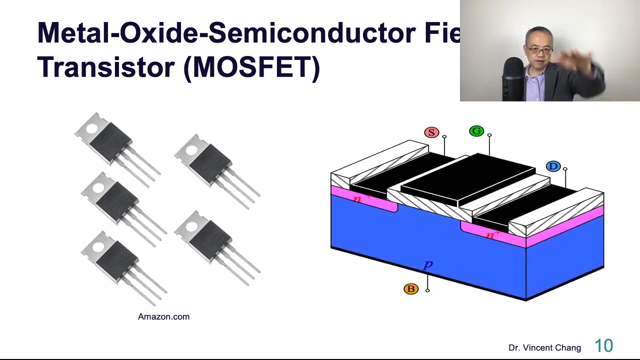 In the MOSFET. just read this: Metal Oxide Semiconductor Field Effect Transistor. So the second word for this term is called oxide. So superior quality of the oxide from the semiconductor material is crucial, And silicon can meet this criteria. So this device. 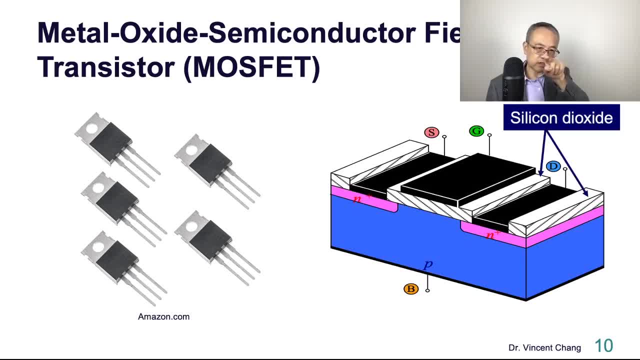 metal. on the top oxide silicon dioxide and the bottom is the p-type semiconductor. So it's the sandwich structure, three layer metal oxide semiconductor MOSFET. So silicon can form a superior quality of the oxide, but germanium doesn't. 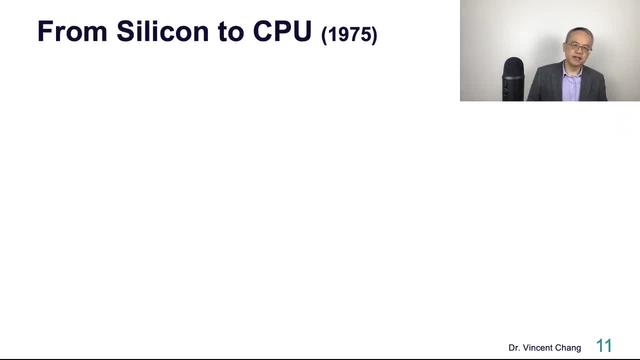 Germanium can't, Germanium can't. Let me tell you a little bit more on this. From silicon to an 8-bit processor, this goal has been achieved: 40, in 1970, 5.. Okay, So this is. 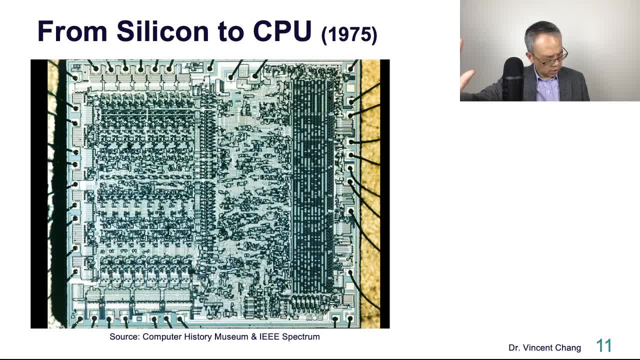 the very famous is the in the cheap Hall fan from the IEEE, So it's from the Computer History Museum. This is the 8-bit microprocessor. It's called 6502, fabricated, produced by a company called. 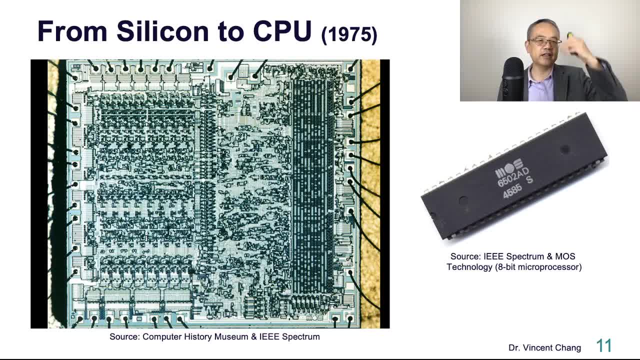 Maas Technology- Again the metal, the reason why they call the Maas Technology metal oxide semiconductor. I just want to emphasize how important it is to have a good quality oxide for a certain type of semiconductor material. I'm still trying to explain. 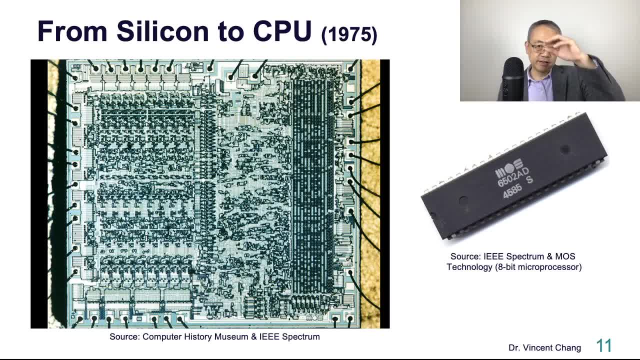 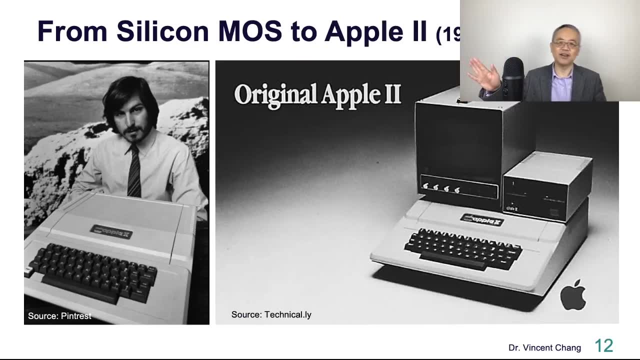 why it's called silicon valley. All right From silicon to a, a CPU, a processor, a 8-bit microprocessor. You know which computer used this processor? The very famous one. All right From silicon Maas. 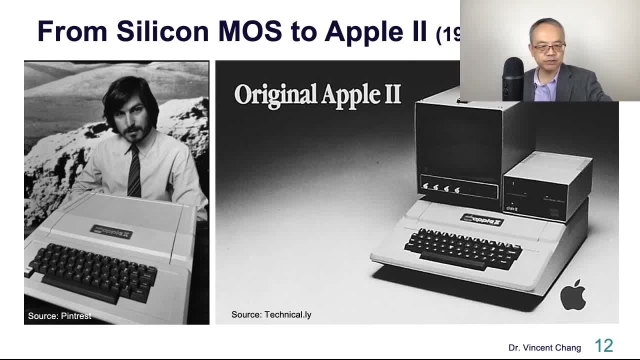 From silicon Maas to Apple II in two years, In 1977.. So this Apple II is powered by the 6502 processor and the underlying technology, silicon Maas technology. All right, Let me tell you another one. 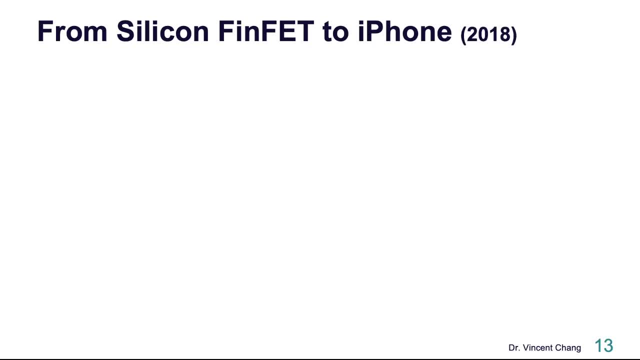 iPhone. Let's fast forward for 41 years, From 1977 to 2018.. All right, iPhone XS came out From silicon FinFET to iPhone. This is on the left-hand side- is the. 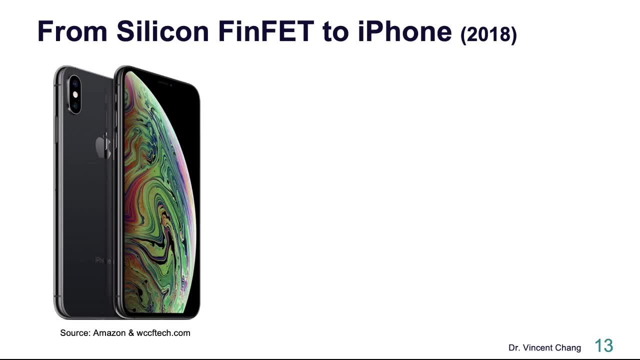 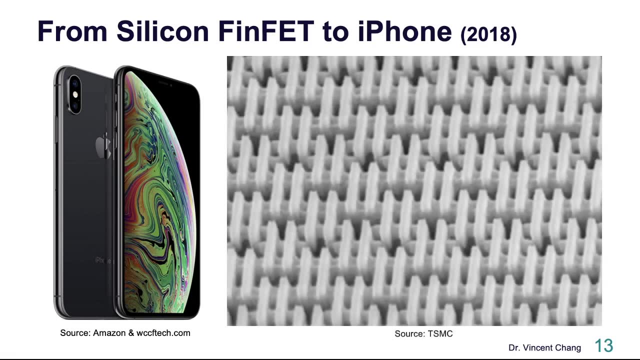 iPhone XS was launched in 2018.. The underlying technology for this is the silicon FinFET. This is the seven nanometer FinFET. Again, the FET is the field effect transistor. The FinFET is: 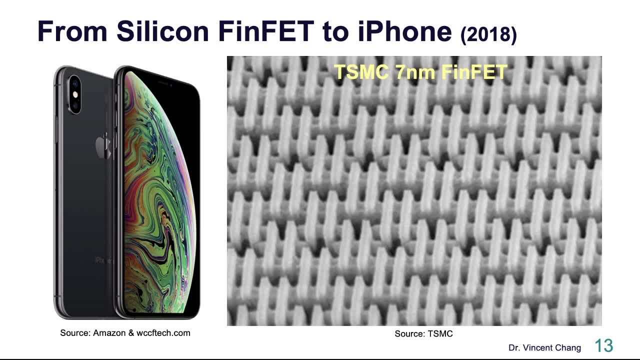 turn the two-dimensional, two-dimensional, two-dimensional, two-dimensional MOSFET into the three-dimensional one. It's a FinFET. It's invented by the two professors at UC Berkeley, So this is fabricated. 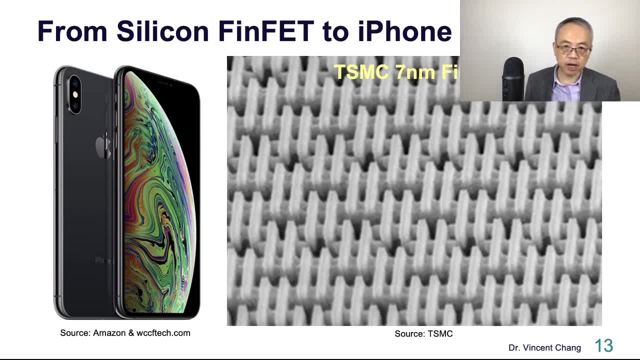 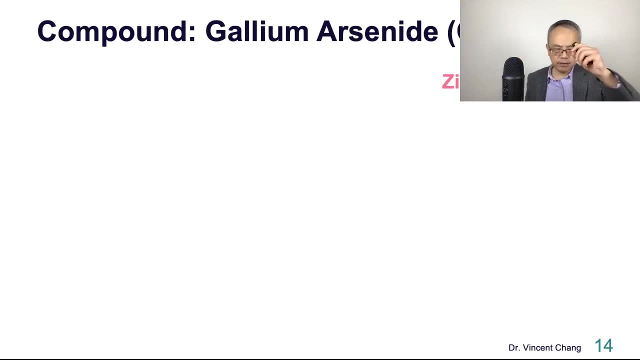 by the Taiwan Semiconductor Manufacturing Company TSMC Seven nanometer FinFET technology. Again, the underlying technology is silicon fin fat- still silicon, silicon fin fat. and then let's move on to another type of material called 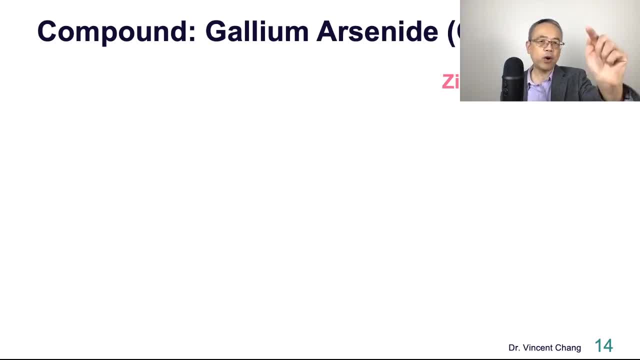 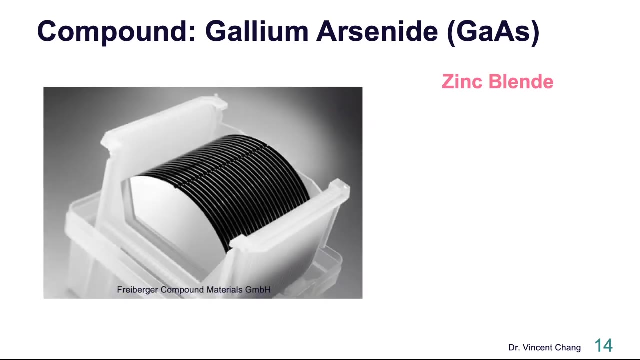 compound semiconductor. let me give you one example: gallium arsenide. gallium arsenide, the crystal structure. crystal structure of the gallium arsenide is zinc blend. on the left hand side is the gallium arsenide wafer. on the right is this crystal structure? 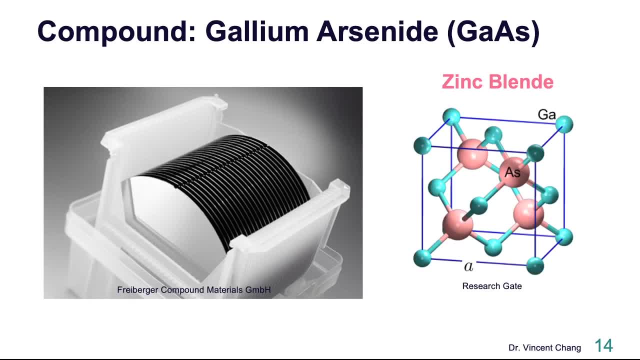 so still, it's the two phase center qubit. but one phase center qubit is from the gallium and another FCC phase center qubit is from another atom called arsenide. so it's the two FCC compound together: gallium, arsenide. so what's special about this? 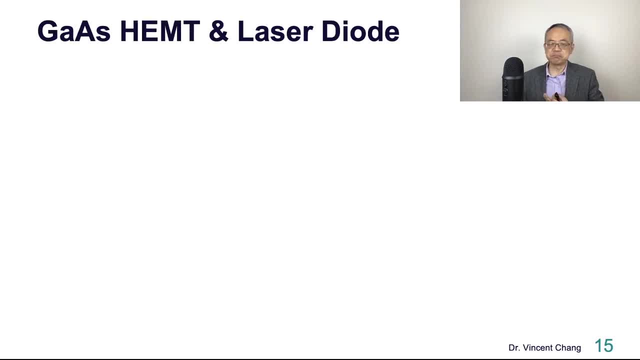 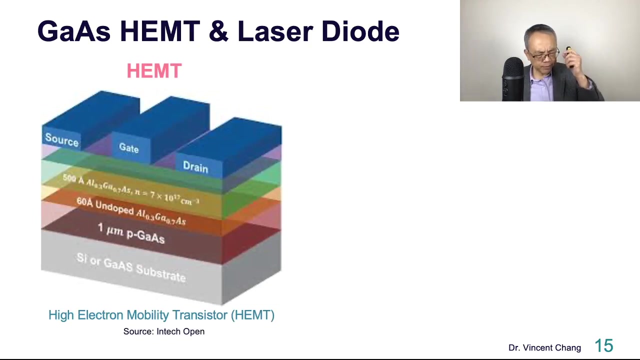 can silicon do everything? can silicon do everything? no, the gallium arsenide has two things that silicon is short of. number one: electromobility- gallium arsenide. gallium arsenide has a very high electromobility for silicon. I remember it's the 1300. 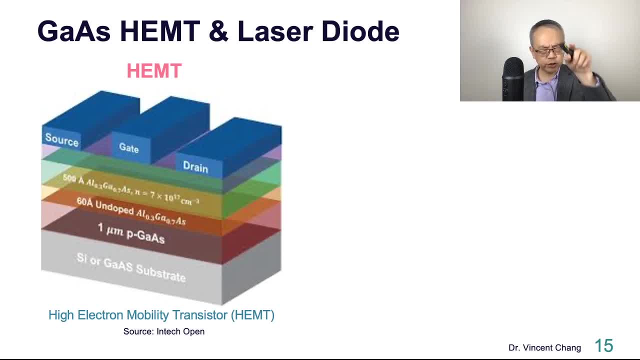 but gallium arsenide can reach to 8000. so which is around around how many times, six times higher than the silicon. so when a material have a higher the mobility, the, the electron can move faster than means what High speed. So see, this device is called HELMT. 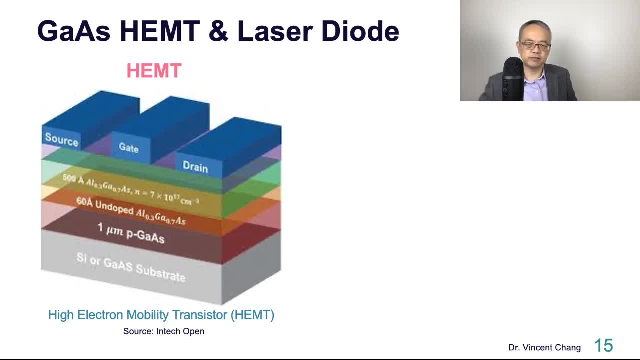 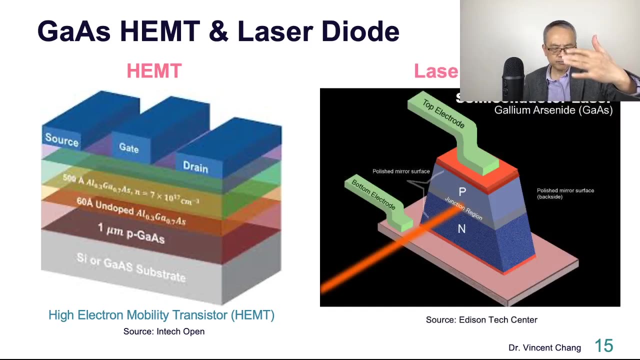 It's called High Electron Mobility Transistor. High Electron Mobility Transistor, It's the high-speed transistor gallium arsenide. The underlying material is gallium arsenide, But on the right-hand side, if you study deeper about the so-called band structure. 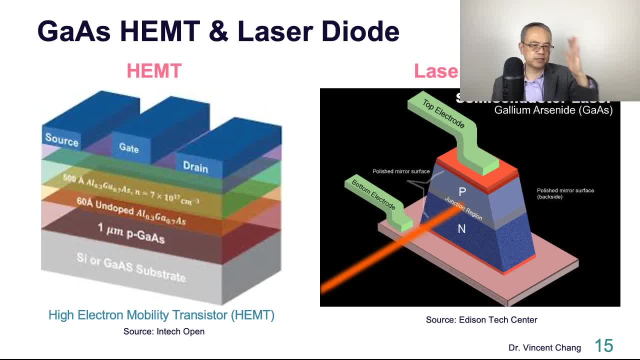 and the NH band structure, and then you will know: the silicon is the indirect band gap material, But for the gallium arsenide it's direct band gap material. So optoelectronics, laser dial, So for the gallium arsenide. 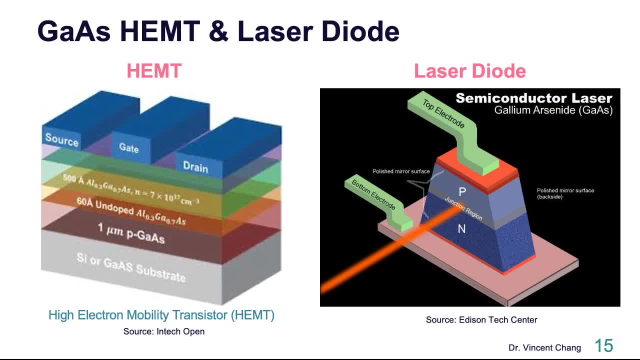 you can produce the laser dial opto-semiconductor laser from gallium Arsenide. It's a laser dial semiconductor laser from gallium arsenide. So two important characteristics compared to the silicon. Number one: very high electron mobility. 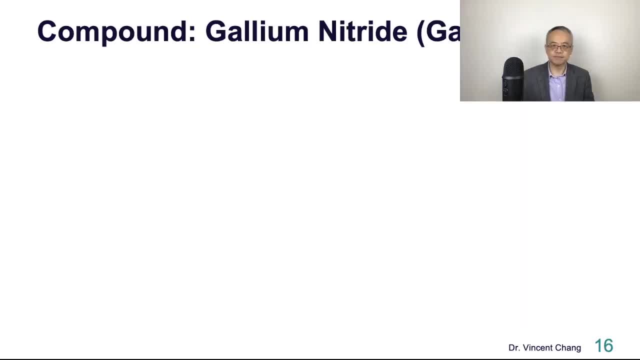 Number two: optoelectronics. Optoelectronics: Let me show you another compound called gallium nitride, Gallium nitride. So for the gallium nitride on the left-hand side is the gallium nitride technology. 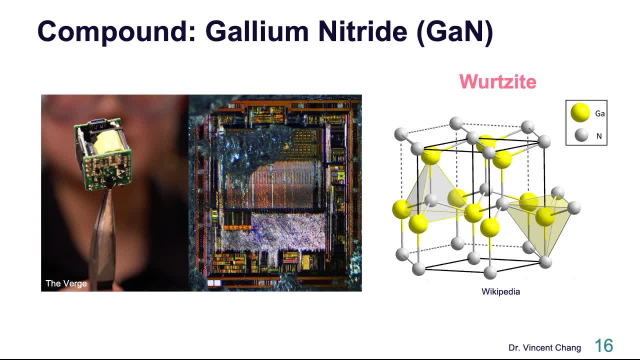 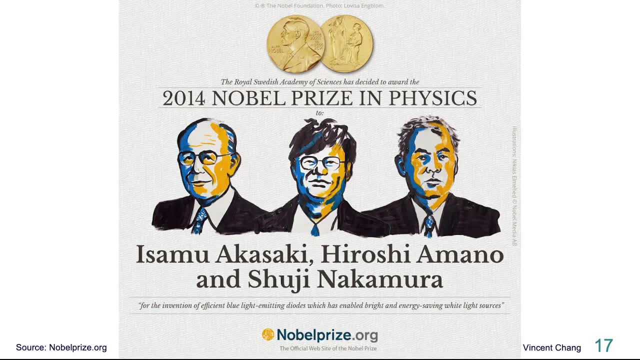 It's called Wurzite. This is the crystal structure. The yellow one is the gallium atom. The white one is the nitrogen atom. When it comes to the gallium nitride, it's inevitable to mention these three gentlemen. 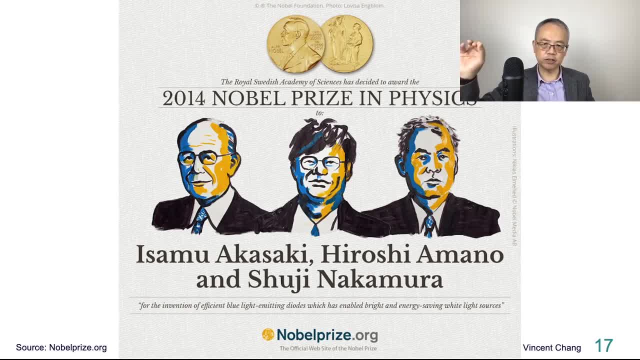 Isamu Akasaki, Hiro Amano and Shuji Nakamura. These three gentlemen won the 2014 Nobel Prize in physics. Why? Because the light-emitting dial, The blue light, for the invention of the blue LED. 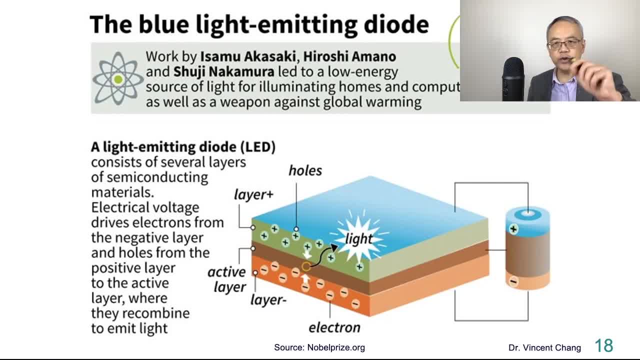 the light-emitting dial, The blue LED. basically, let me just quickly teach you this. This is the P-N junction dial, The first. the top is the hole. The majority carrier is hole On the bottom. the N is the electron right. 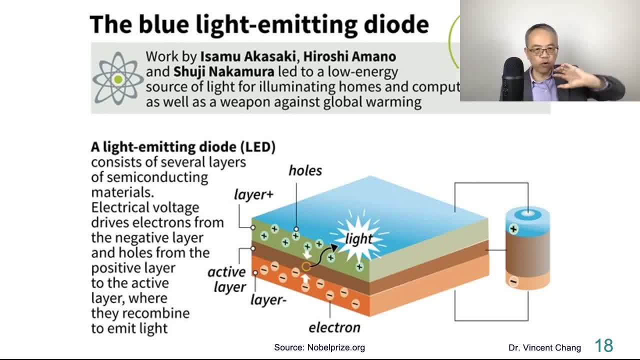 So when you forward bias a dial, When you forward bias a dial, then the hole and the electron will meet at the junction And then, when they meet together, they recombine, They join. When they join, they recombine. 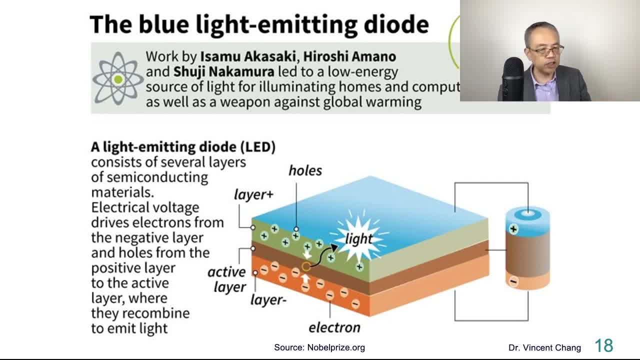 you will release the energy And then the energy will turn from, will be converted from the electron energy, electric energy, to the optical energy And the spectrum of that energy. if you learn the modern physics, E equals h, mu, Planck, constant times, the frequency. 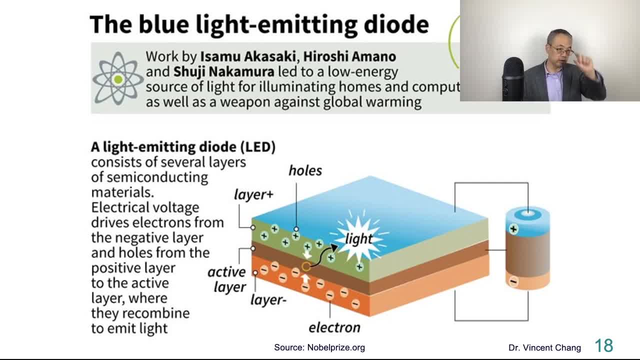 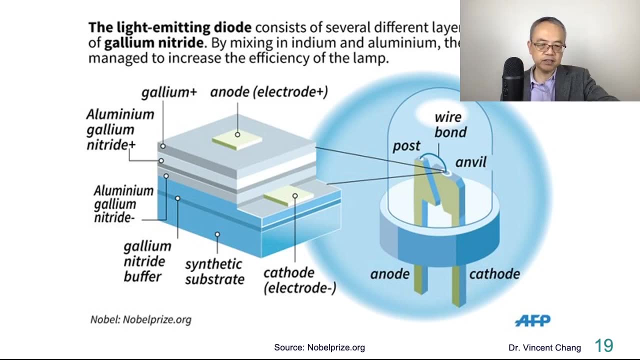 Then you can calculate the wavelength. It falls into the blue light wavelength. So this is the blue light-emitting dial And these three gentlemen. the light-emitting dial consists of the several different layers of gallium nitride. It's from the gallium nitride.